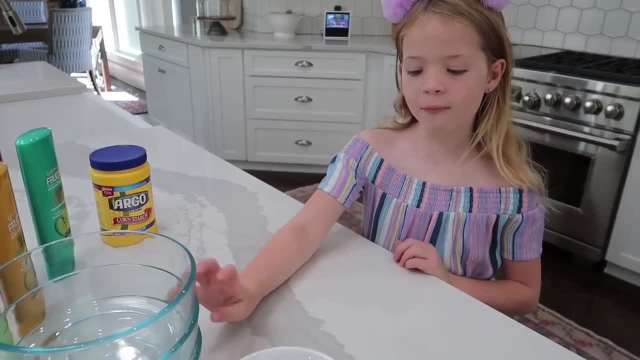 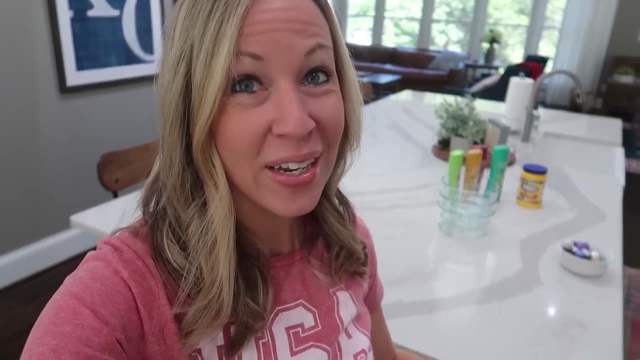 And some cornstarch And A cup of bowls and some food coloring. That's right. The basic recipe's really easy. All you need is conditioner and cornstarch. You can add food coloring if you wanna add some fun colors though. 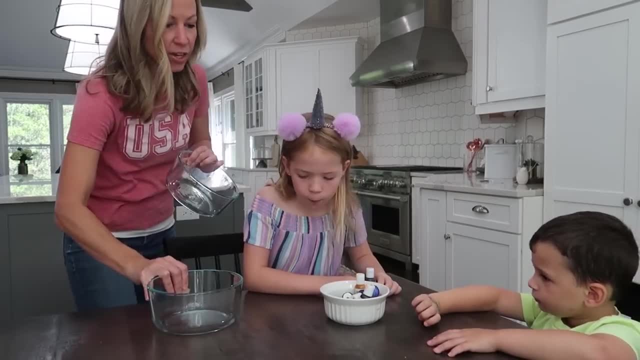 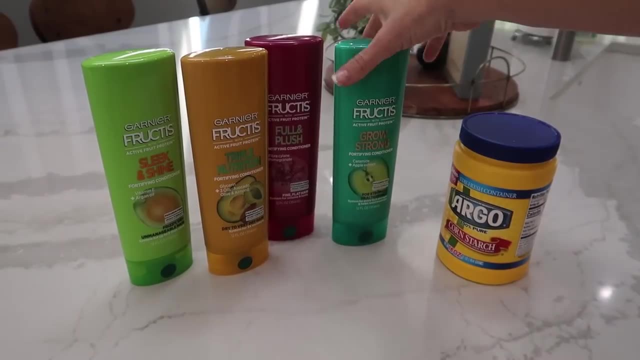 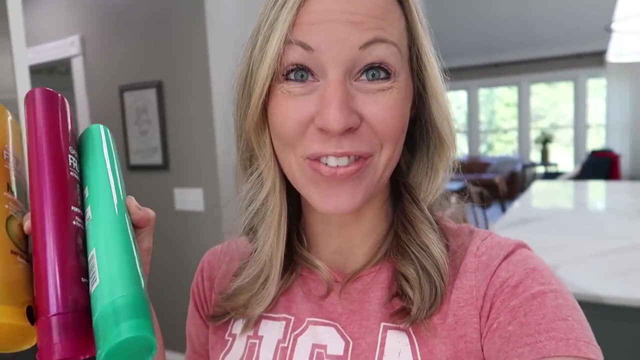 Should we do the purple? Alright, you're gonna get your own mixing bowl. Oh, you get to choose yours. This is red, This is mine. I got a variety of conditioners. You really only need one kind, but I thought it would be fun to get some scented. 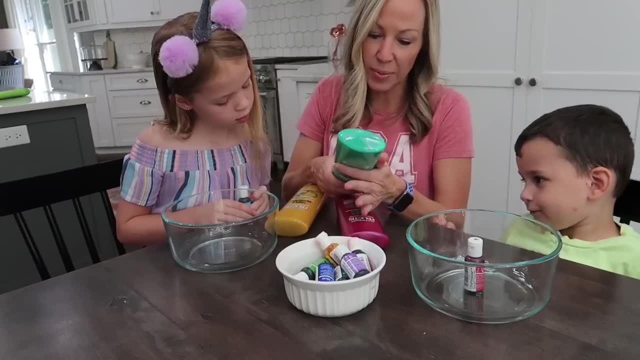 versions so the kids could pick out the scents they like best for their cloud dough. This one has like an apple smell to it. Can I smell Mm-hmm? Can I smell Apples? You wanna smell the apples? Is this lavender? 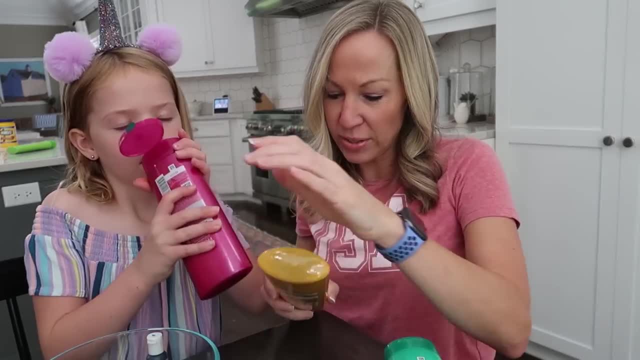 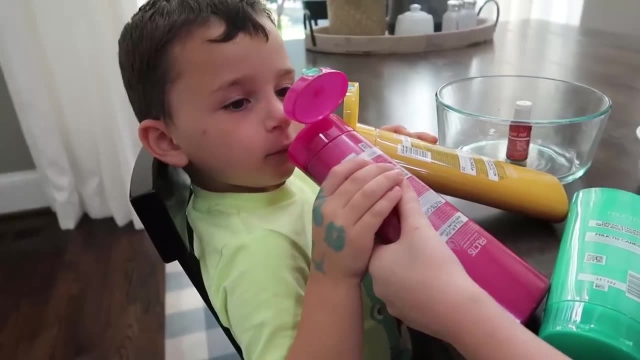 And this one is like pomegranate. And then we also have one that has like some oils like avocado, olive and almond Smells good too. a little cleaner though, I wanna do the pink one, because that smells super yummy. 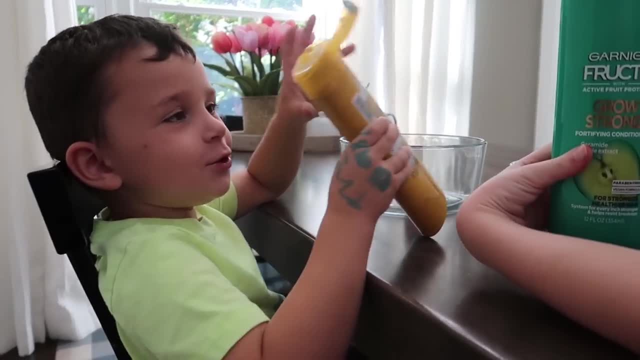 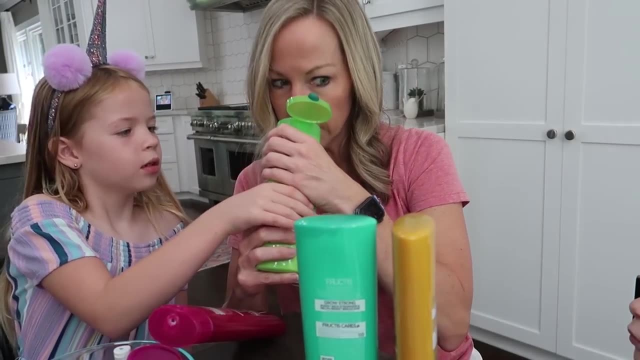 That's pomegranate. I wanna eat it. What one do you wanna do This? That one, Okay, That's a good one. That's a good choice. I actually forgot this one too. This one is vitamin E and argan oil. 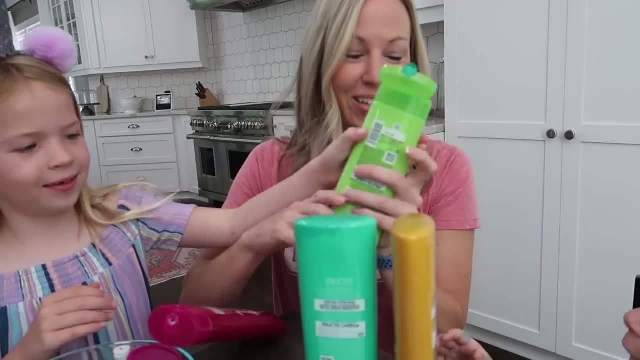 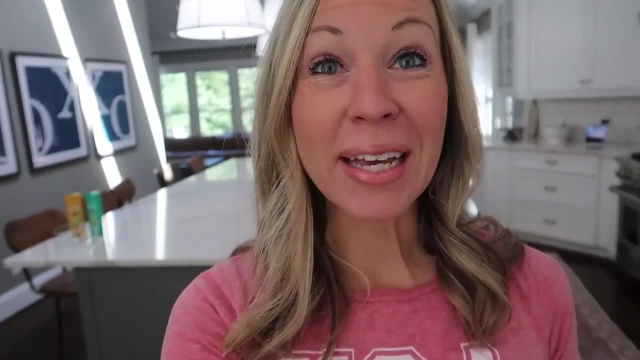 This smells good too. It smells very fresh and clean. Can I smell? You wanna smell it? You wanna do this one? Yeah, you like that one. So the first thing you do is mix two-part cornstarch with one-part conditioner in a bowl. 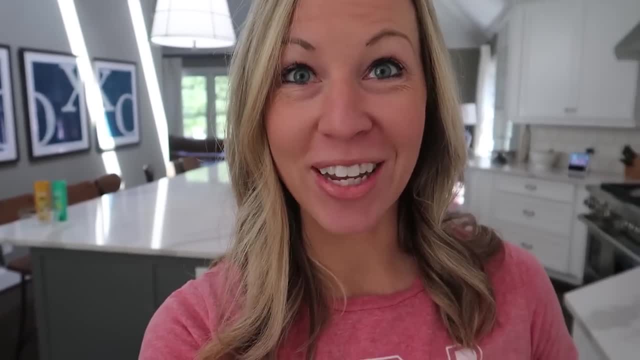 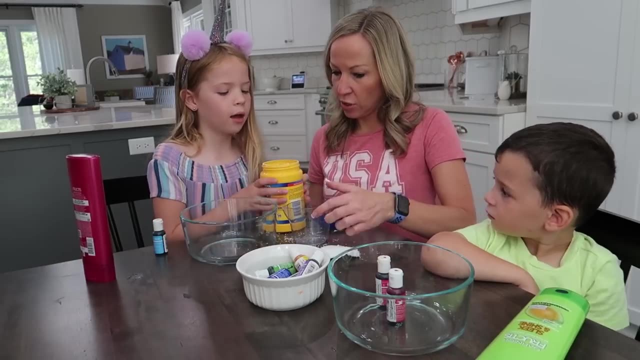 So we're gonna do two cups of cornstarch with one cup of conditioner. Here's our cornstarch. It's a little bit messy, Whoa, And we're gonna do two cups. We're gonna fill it up to the one cup mark twice. 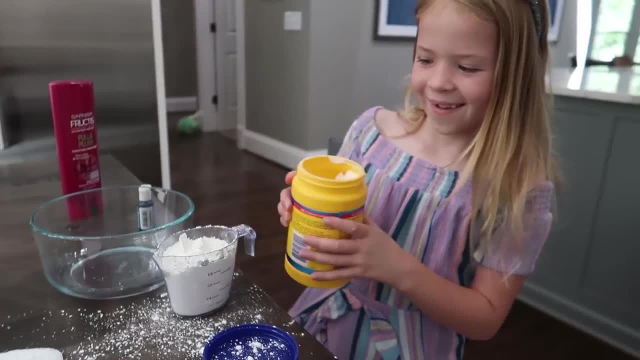 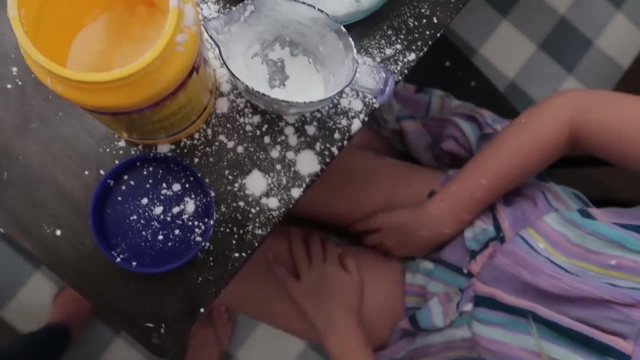 Whoa, It's a little messy, isn't it? Yeah, Whoa, There's probably a neater way to do this than what Maya just did, but we'll make it work. I think Maya's covered with cornstarch now. 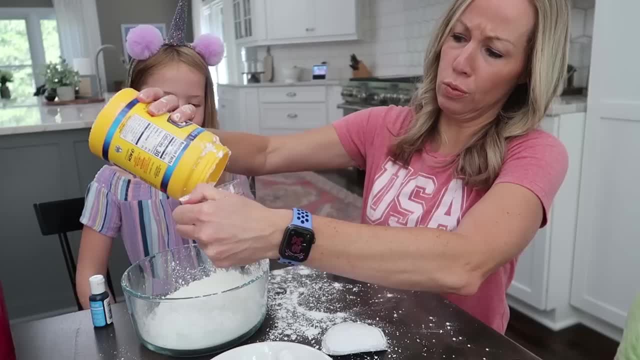 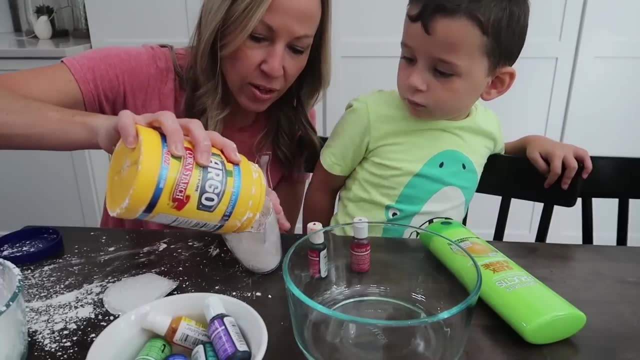 All right, let's do another cup, because you need two cups for it. I'm gonna do this over the bowl. I didn't think it would be this messy. That's about two cups Ready. We're gonna do one cup. I can do this. 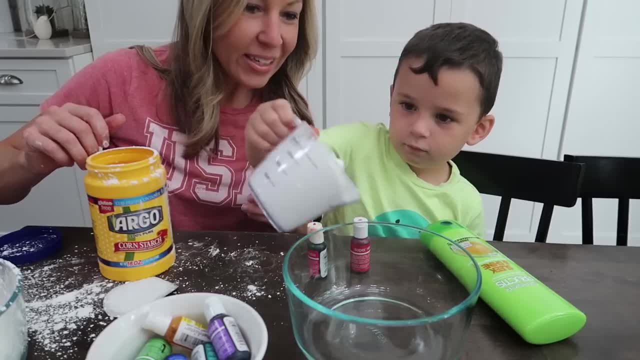 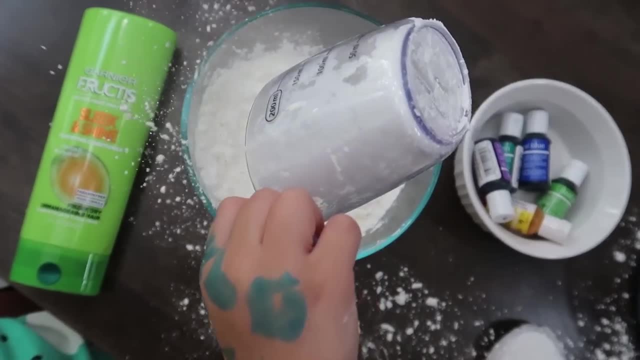 You can pour it for me. You wanna do that for me? Yeah, Really, gently, Whoa Good job. Tap it And we do one more cup. And now that we have two cups of cornstarch in each of their bowls, we're gonna add one. 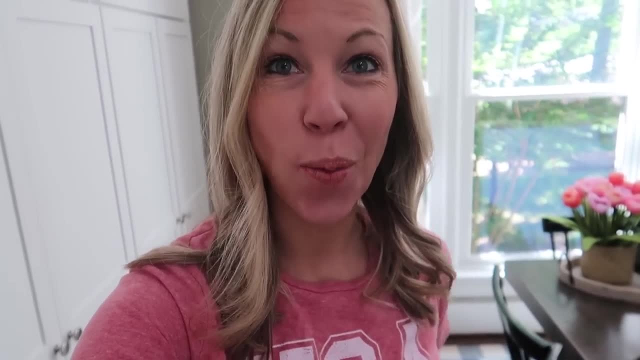 cup of conditioner to each bowl. I think you're making a mess, Colin. I think this might be a good time to go ahead and mix the food coloring with the conditioner. Okay, Okay, Okay, Okay, Okay, Okay Okay. 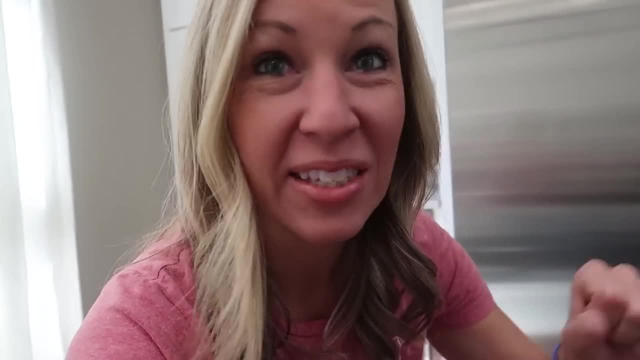 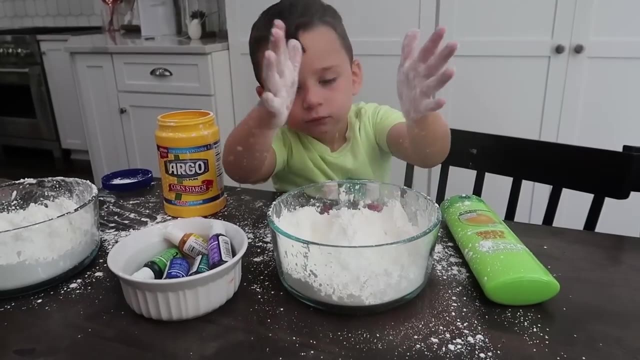 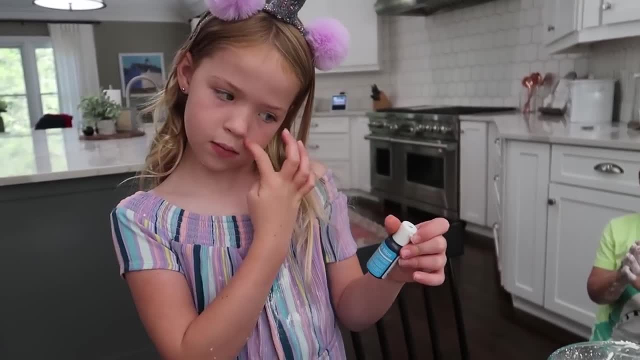 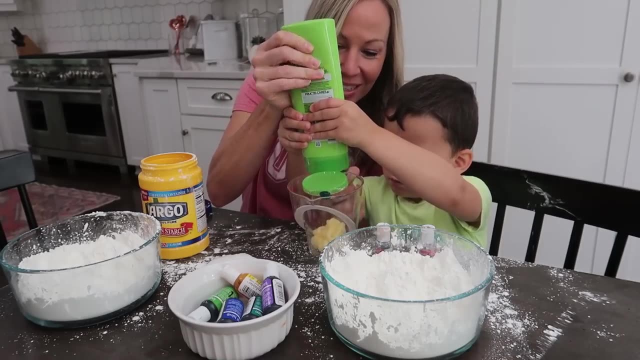 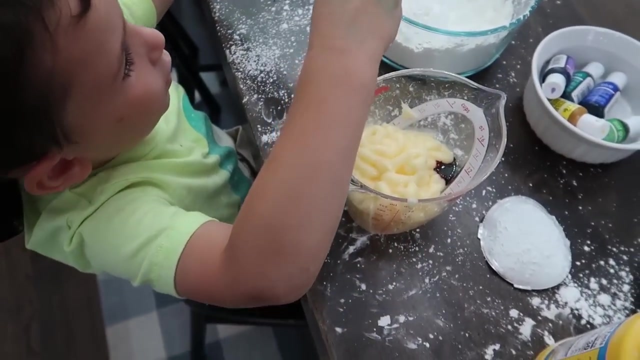 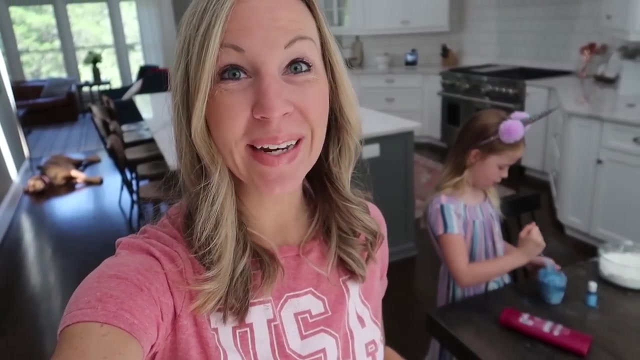 I'm adding some sky blue, Sky blue. Whee, Yours is yellow. Your conditioner has a color to it. What color are we gonna add? Oh, I think Colin's choosing red. Yeah, Yeah, the conditioner. we're going to add it to the bowl where we already have the cornstarch, and we're 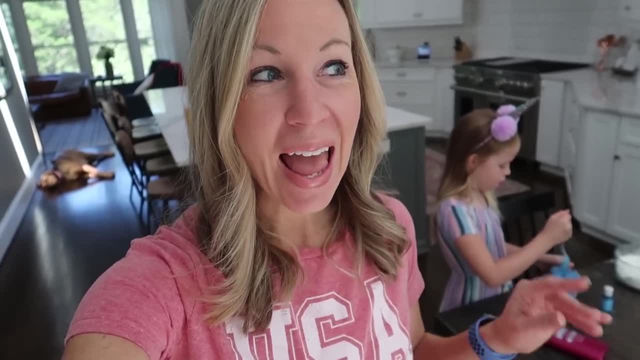 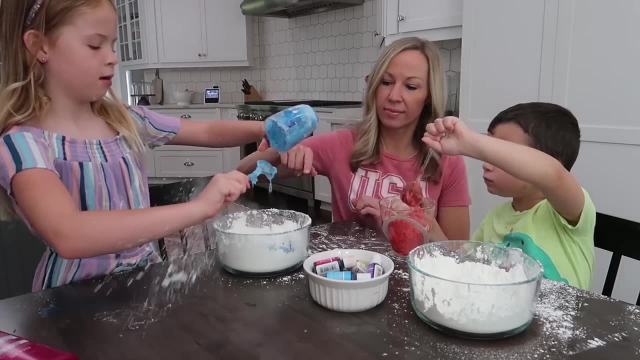 going to just knead it with our fingers until it gets to a good consistency. it should be kind of like a play-doh kind of like a slime, kind of somewhere in between. you do this calm like. you turn it upside down. yeah, oh, put it close to your ball and you can get your hands in there. and 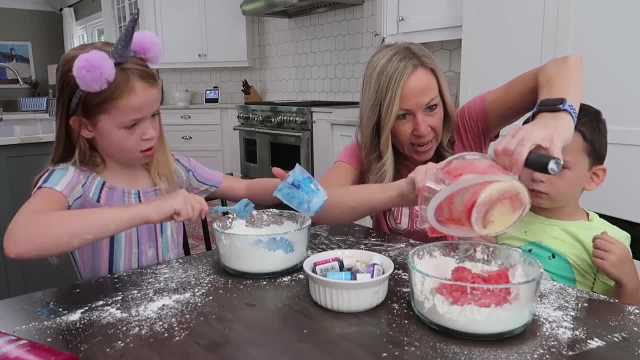 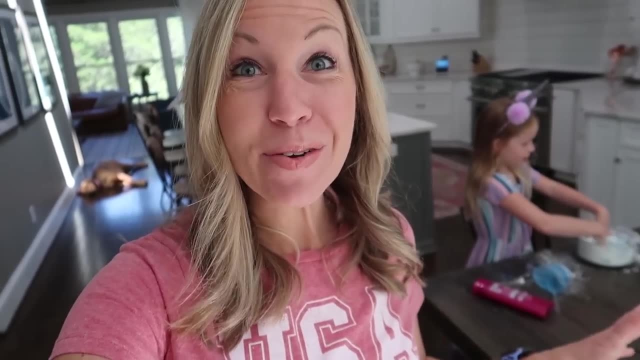 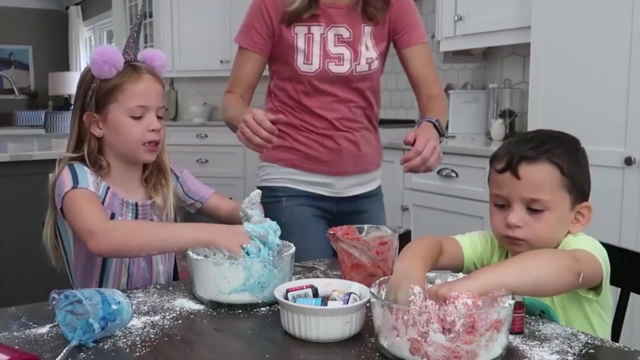 you're gonna mix it really well and you're gonna knead it like you're kneading dough. while they're busy mixing, i'm gonna get on mess control and kind of get a little bit of this mess picked up. i did not think it wouldn't be this messy to make this feels so good and keep on mixing until it's not sticking. 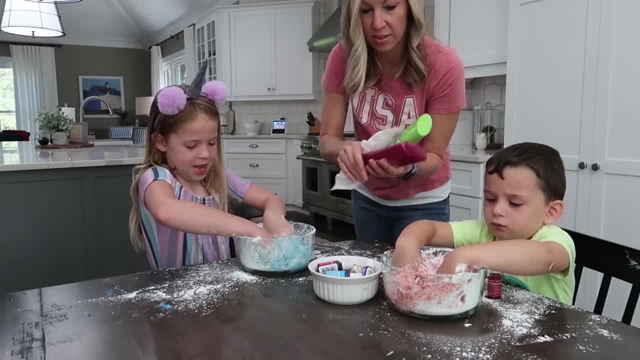 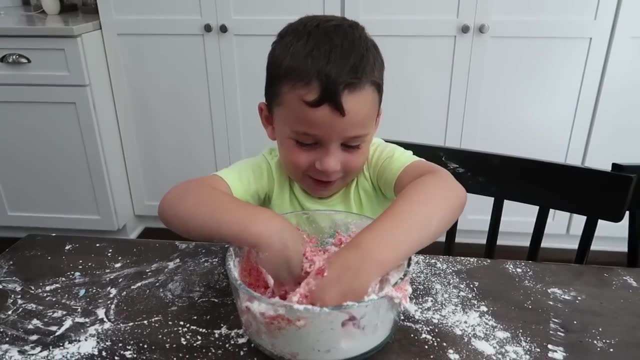 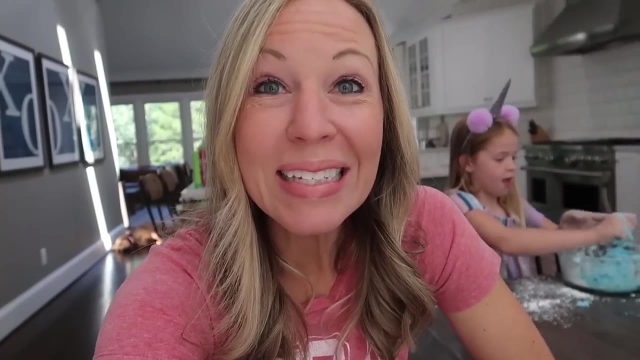 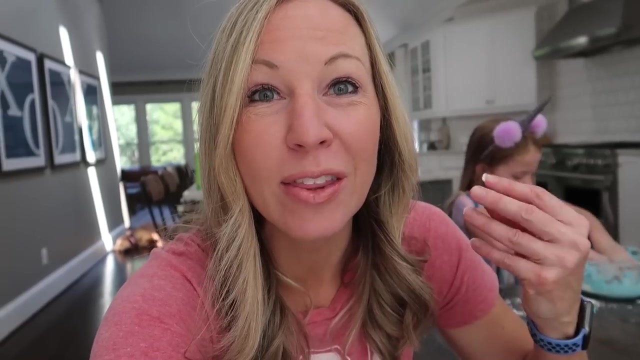 we have cornstarch everywhere, guys, everywhere, absolutely everywhere. i decided to make this today because colin's preacher school teacher actually recommended it. She said it's great for developing those fine motor skills and really getting those muscles in your fingers and your hands stronger. 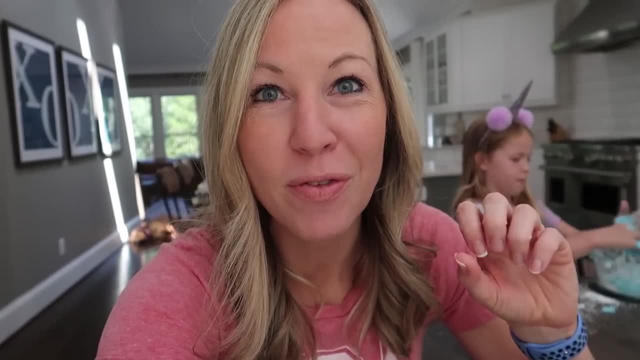 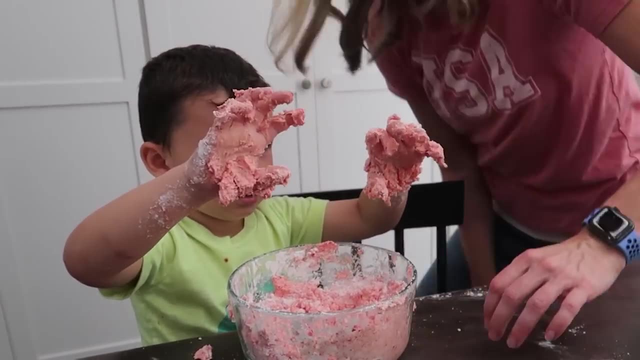 It's kind of the step before Play-Doh. So this is kind of warms them up before they move on to Play-Doh play. I don't want this sticky on my hands. You do need some help, Colin. Yeah, I'm gonna help Colin get his form. 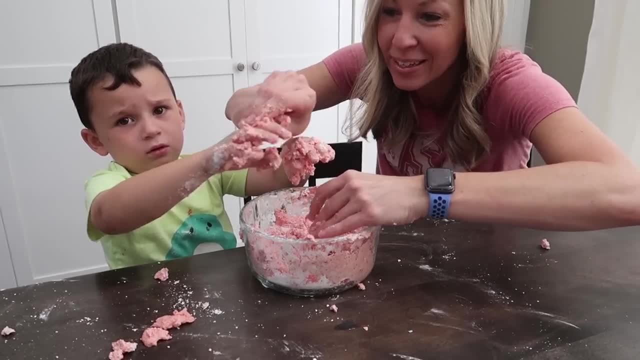 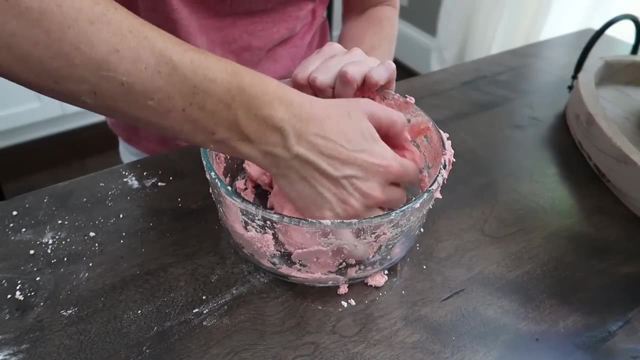 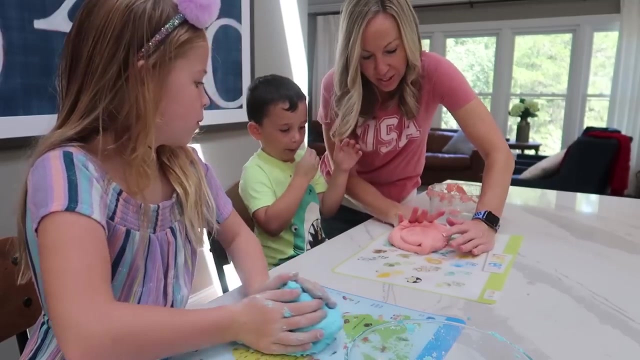 so that he can move on from the creation stage to the play stage. Let's really work on kneading this. Let's do it. Ooh, Now here we can really knead it a little bit more. Oh, that feels good. 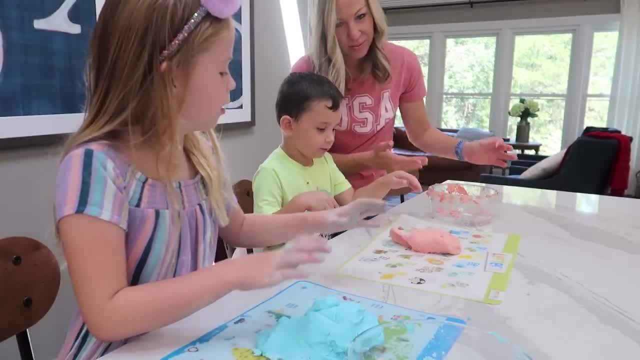 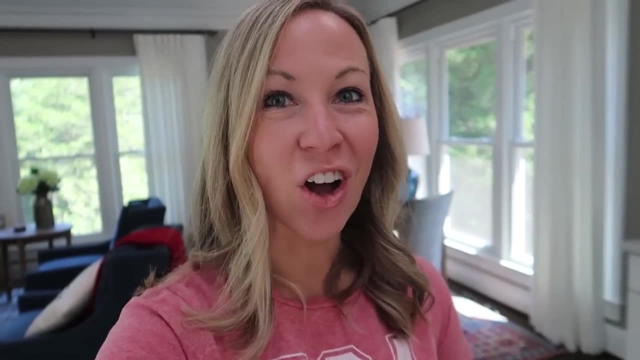 Do you want to put your hands on there? There, Ooh, This is so much more fun than before. What's interesting is the consistency of Colin's and Maya's Cloud Dough is very different. I think Maya's is more how Cloud Dough is supposed to feel. 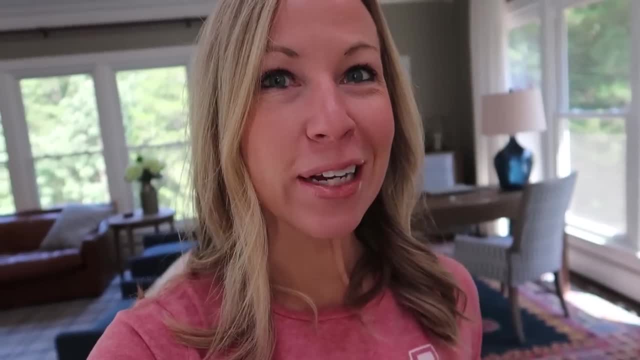 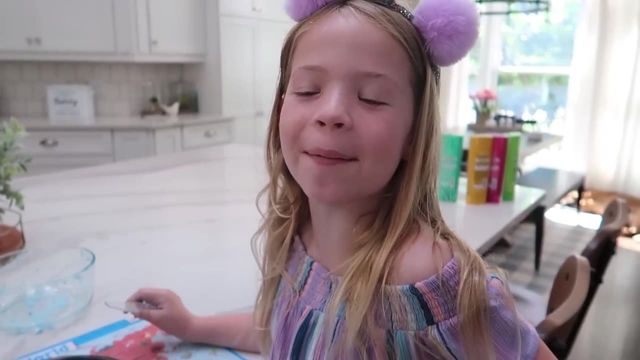 and Colin's is a little bit stickier, So I think maybe more of his ingredients ended up on the floor than in the bowl, but I think he's still having fun playing with it. I forgot about the scent, and then, when Colin showed me it, 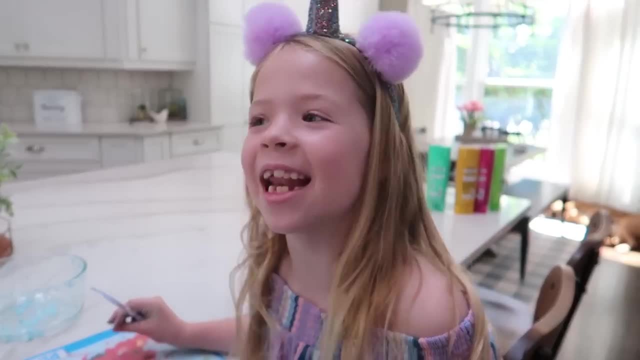 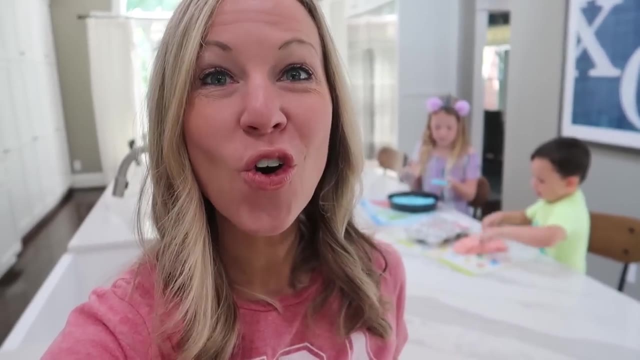 he was like: smell it. I'm like, oh yeah, the scent. It smells so good. I'm glad I decided to add in some real kitchen items that I have around the home for them to play with with their Cloud Dough, because I often find 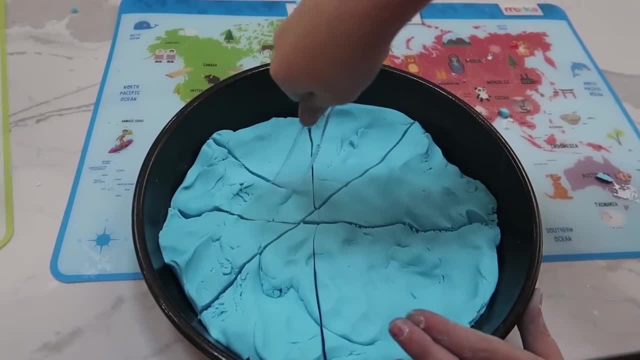 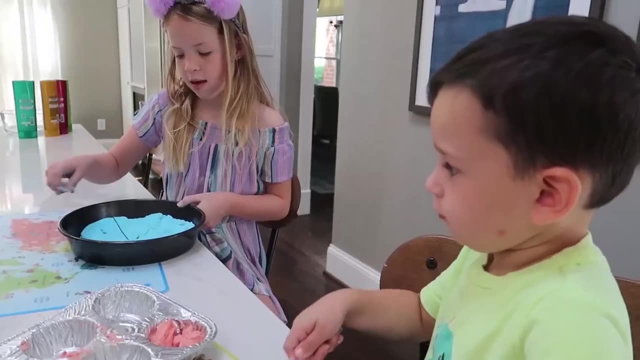 if I buy toy sets of kitchen materials, the kids never have as much fun with them as they do with with the real stuff. So we're pulling out some real stuff from the kitchen for them to experiment with. Look, I made a cake. 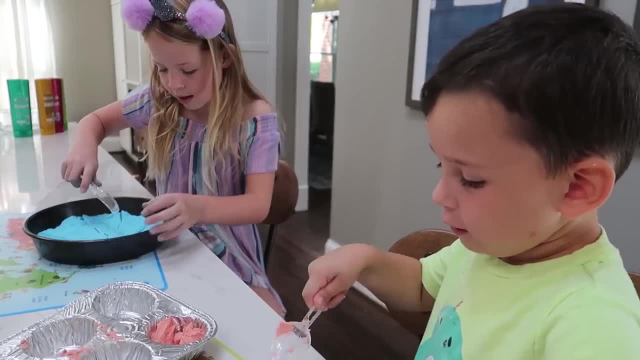 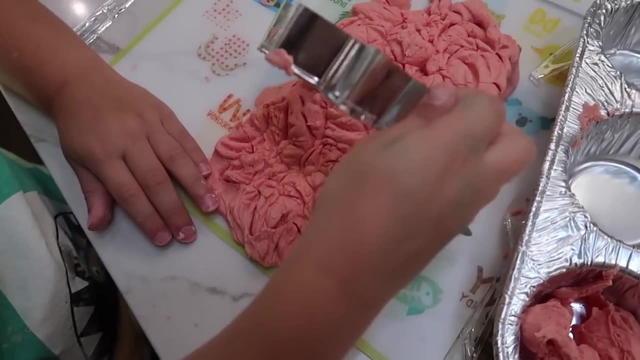 Make some muffins for me, and I'll give you a piece of my cake too. Okay, I like it. Cookies, Some cookie cutters too. Whoa Yup, I got a little. you know, for me it's very easy to find. 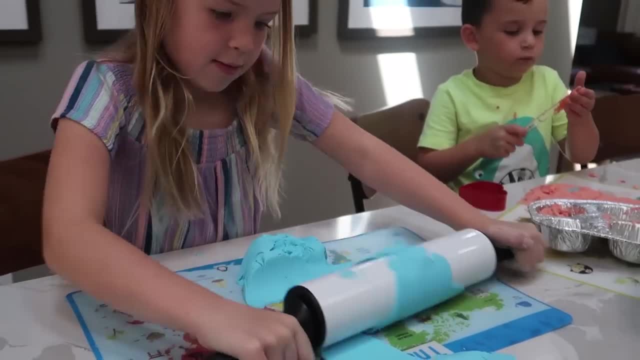 I just have to get the right size. There's four in here. I have three. I'm gonna make one of these. I got the whole set. I got one of these. I'm gonna use this one. I'm gonna use the other one. 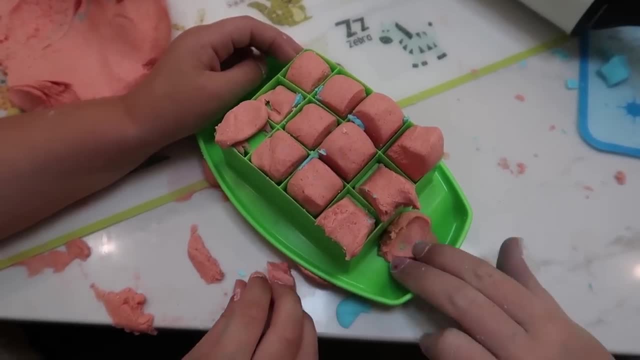 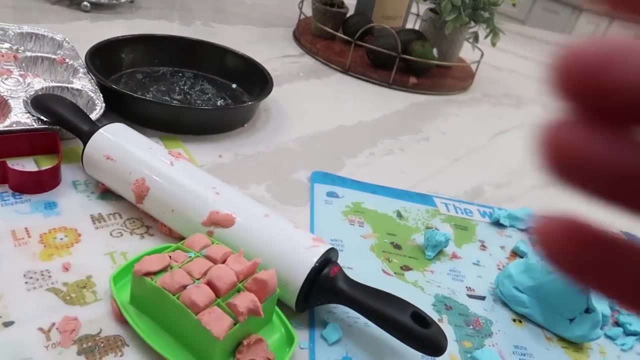 You guys know what kitchen tool this is. It makes sandwiches go into little squares It is. I used to do this for Addy in preschool a lot. It's one of those sandwich cutters and it makes teeny tiny sandwiches. I used to make peanut butter and jelly sandwiches. 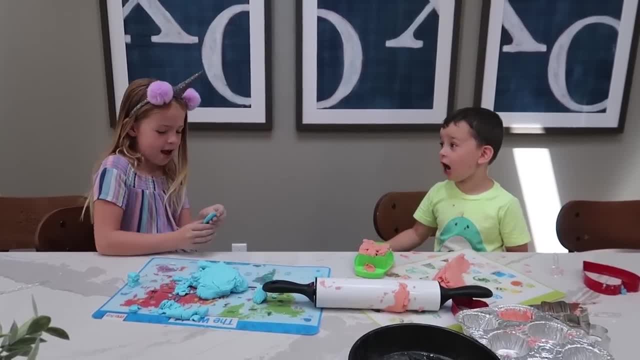 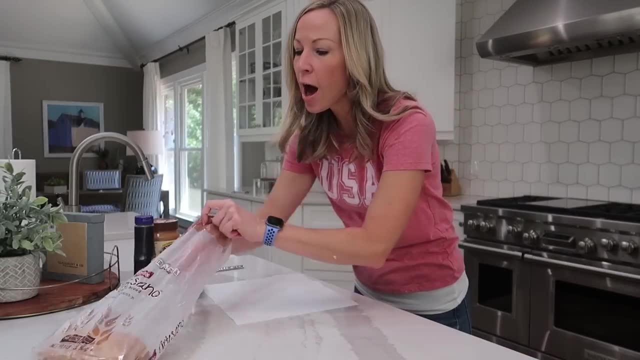 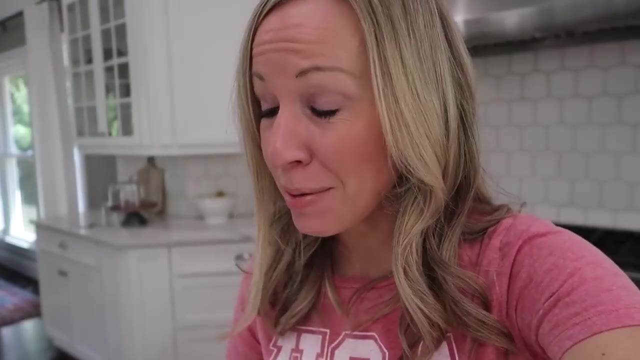 for Addy, like this. Peanut butter and jelly. I'm trying Peanuts, peanut butter and jelly. Peanut butter and jelly sandwiches. Mickey Coming up With all the sandwich cutter talk, it made Maya remember that we have an old Mickey Mouse sandwich cutter. 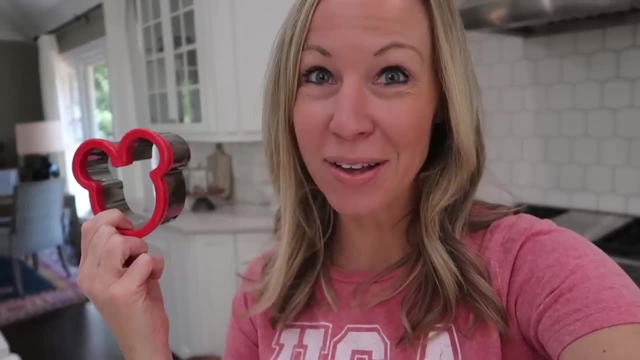 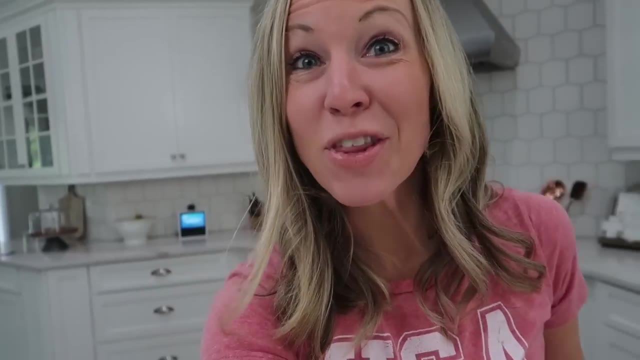 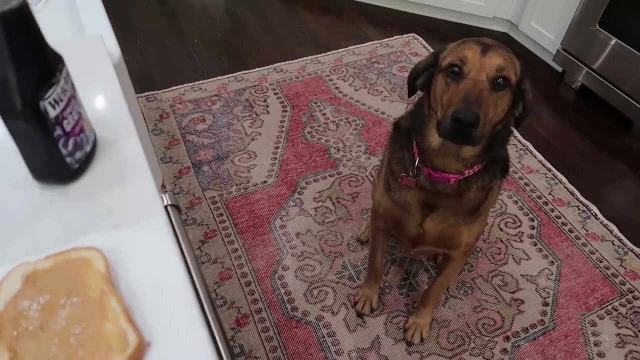 so the kids are requesting peanut butter and jelly sandwiches, Mickey Mouse style, for lunch. Oh, and of course, Sandy came in the room. Oh, no, no, no, I think Sandy smelled the peanut butter. Oh, look at that good dog sitting there. 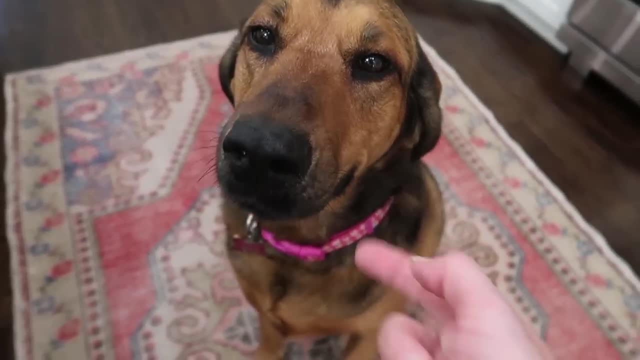 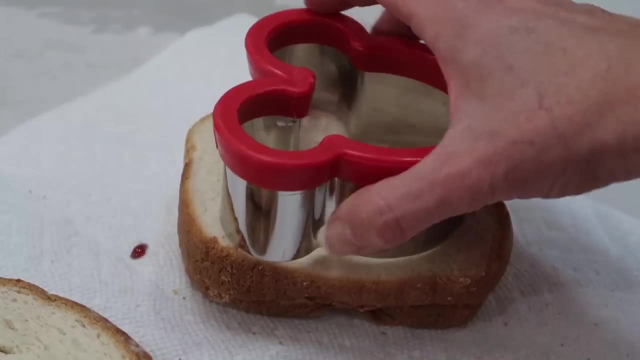 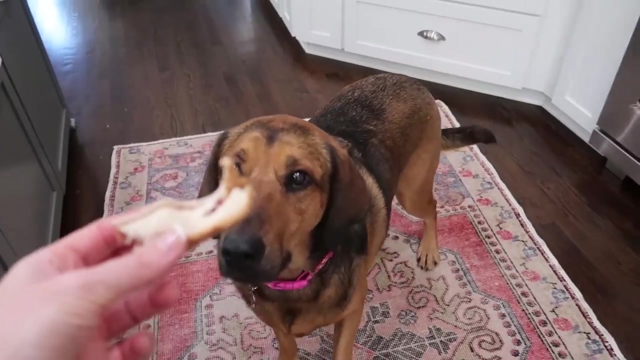 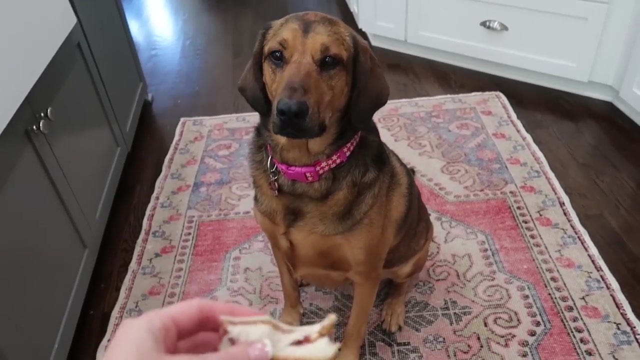 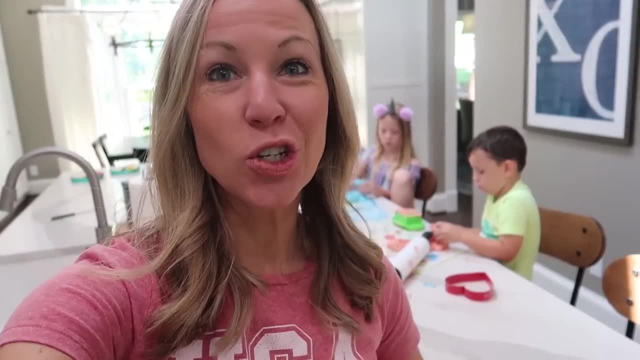 it's really important that you keep it dry and away from air, so it's good to wrap it in saran wrap and then put it in like a zip lock bag for storage If, when you open it, it's a little bit dry. 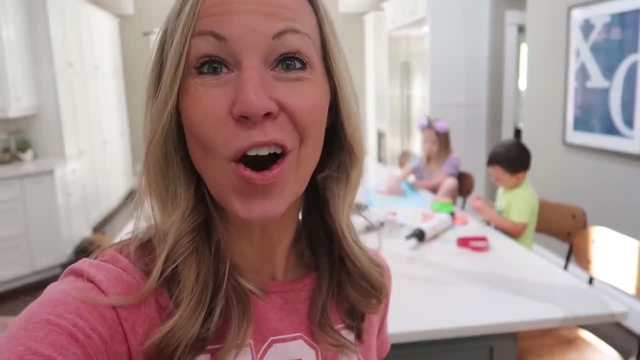 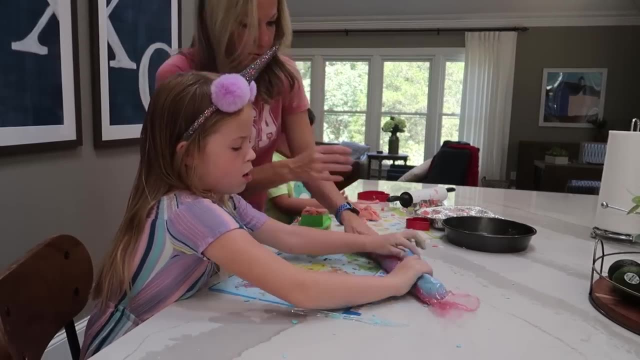 you can just add some more conditioner to it and really knead it, and it should be good to go Put it on there and then wrap it up. Okay, and you can do it like that. Okay, Wrap it up. really well, In general, cloud dough doesn't last quite as long. 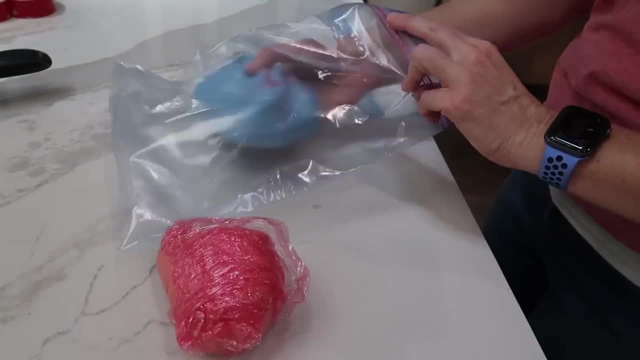 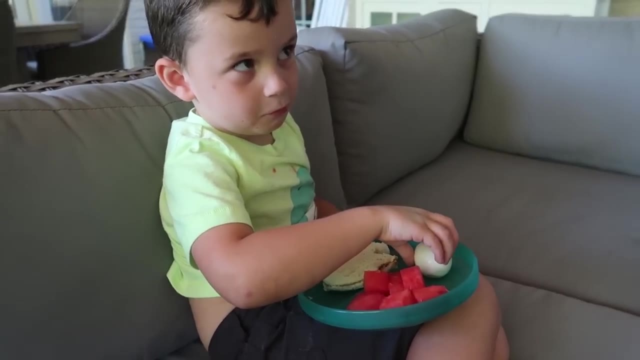 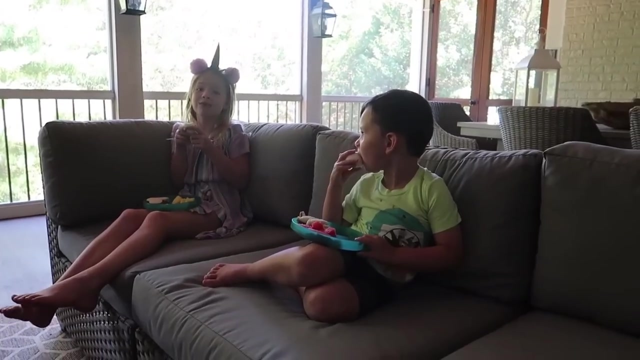 as Play-Doh does. but the good thing is it's really easy to make, so it's easy to whip up another batch if yours gets too dry to use. What's the verdict? Do Mickey Mouse sandwiches taste better than regular sandwiches? Yeah, 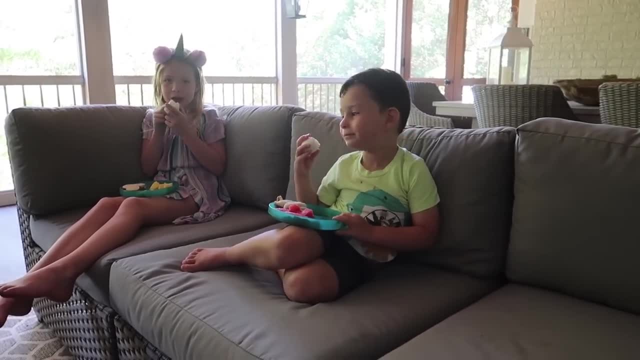 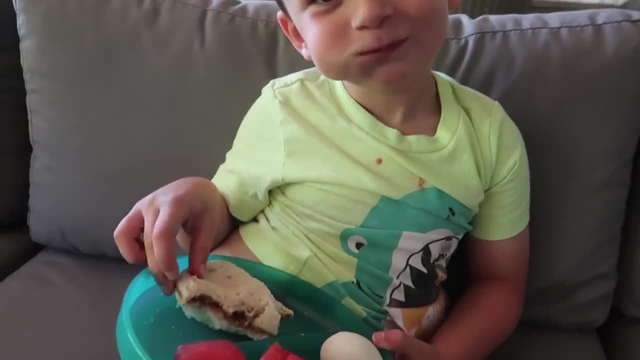 They do. What about you, Colin? Yeah, they do. Well, if you guys could eat sandwiches in any shape, what would they be? Mickey Mouse? Mickey Mouse, You have a Mickey Mouse sandwich, Princess one, A princess-shaped sandwich. 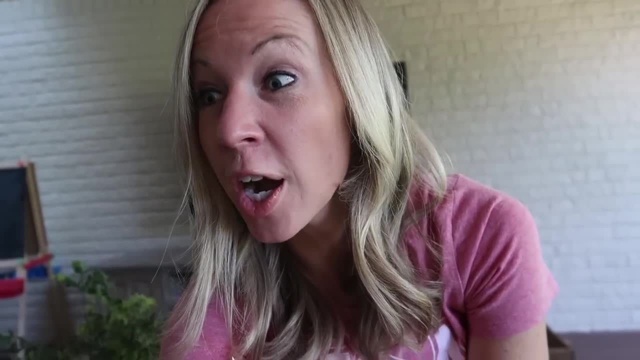 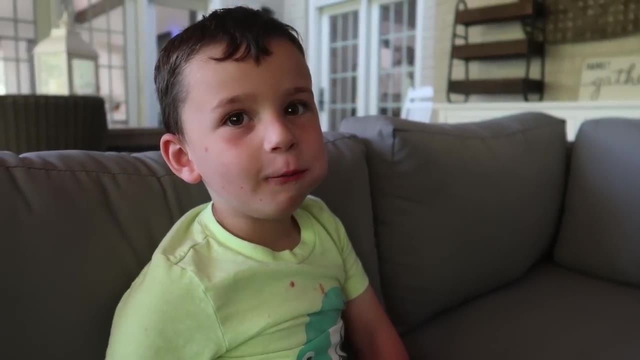 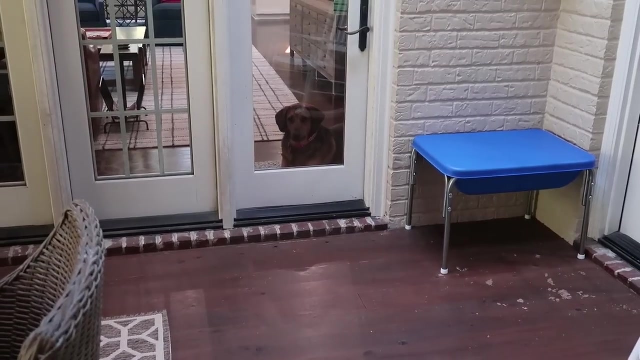 Ooh, Colin, what about a shark? or an astronaut, Spider-Man, Ooh, Spider-Man. What would you want, Spider-Man, Spider-Man? I think Sandy would be happy eating sandwiches in any shape. She's hanging by the door to the Screenton porch. 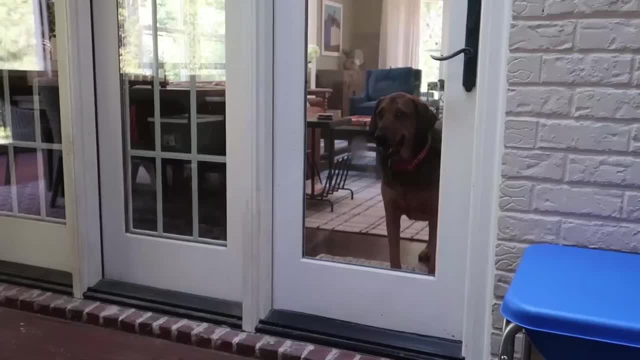 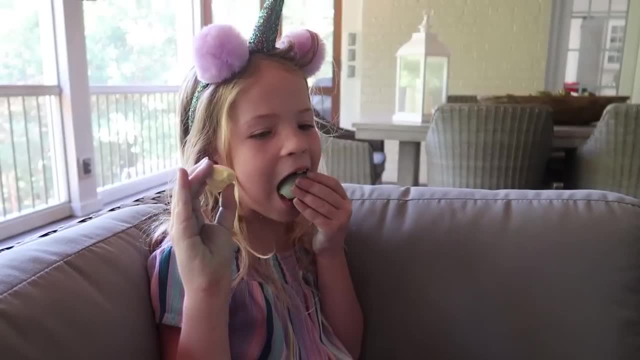 and just pawing at it, wanting to come out and have a bit of a sandwich with us. It was probably a bad idea of me to give her that little scrap of crust, because now she knows how good it is. Our Screenton porch is one of the big reasons. 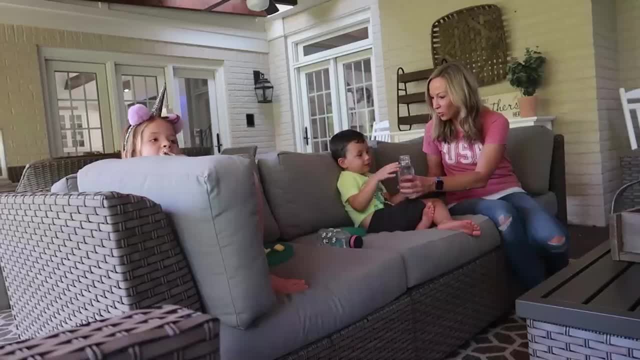 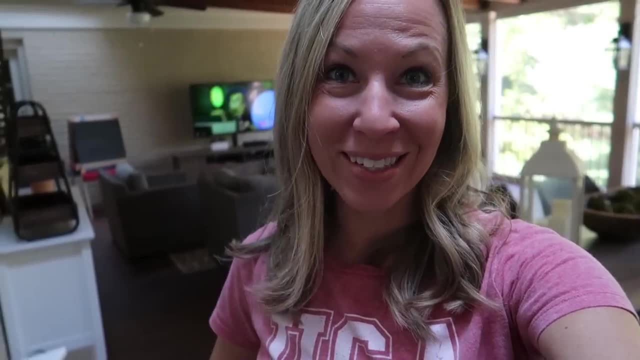 we bought this house. It's one of our favorite places to hang out, eat our meals, like to come out here and work, And we love it so much that we, I think, are getting ready to do something with our porch downstairs. 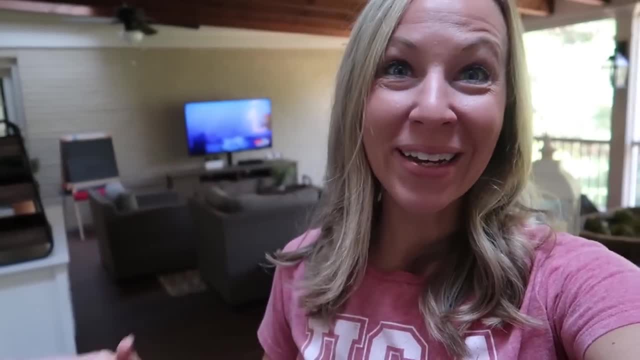 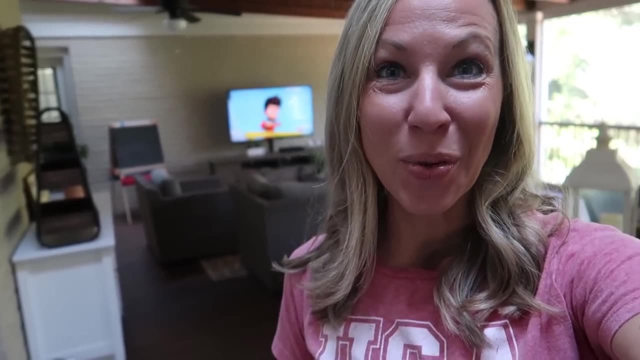 maybe Screenton make it kind of a cool fun environment. But right now the kids have taken over the space and I'm going to show you around that a little bit later, when Addy is done filming for her gaming channel, because they have turned it. 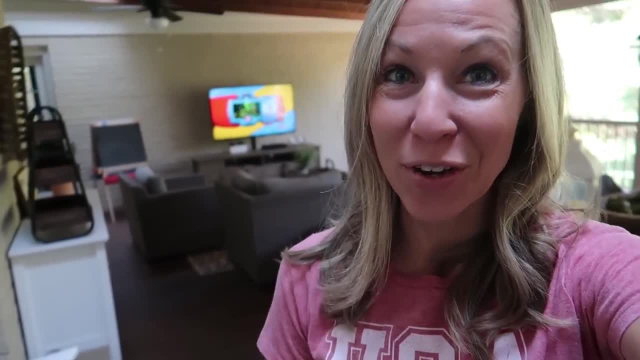 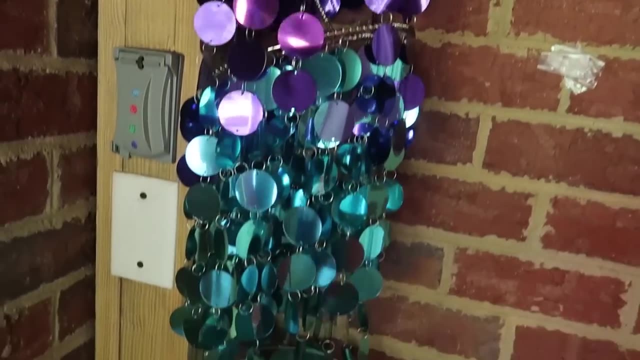 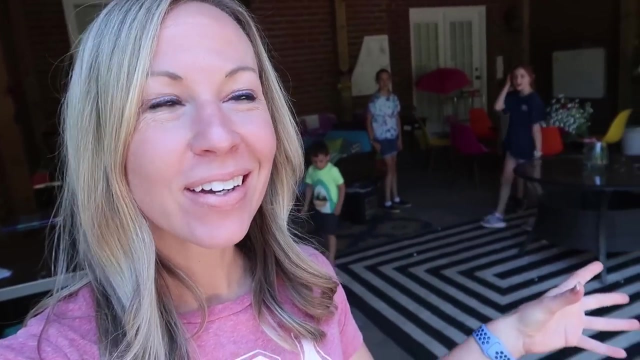 into a crazy fun hideout with all their neighborhood friends. Addy's done filming now so I thought I would come down here to the hideout. do you call it a hideout or a hangout Hideout, Hideout for the kids to show you around. 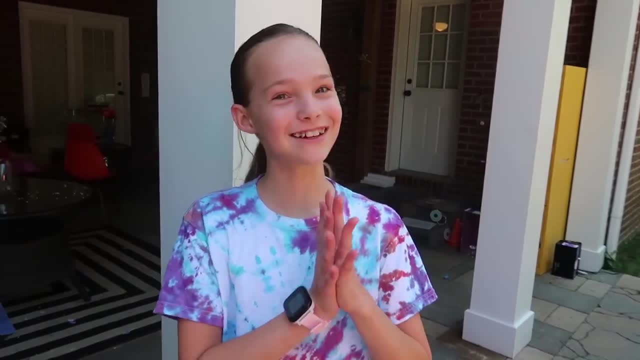 Addy, why don't you show me something in your hangout that you love? Oh, how about we start with the outside porch? The outside porch: Okay, this is your porch area. We can sit and have lunch here. I love it. 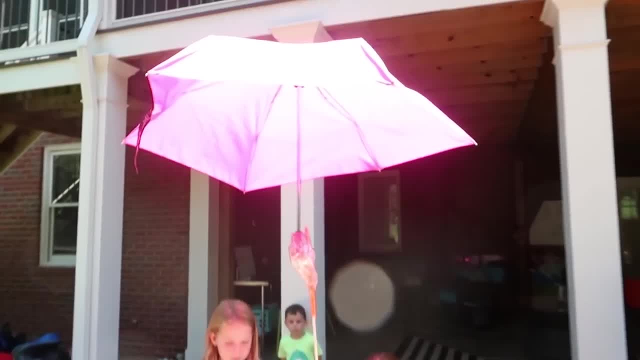 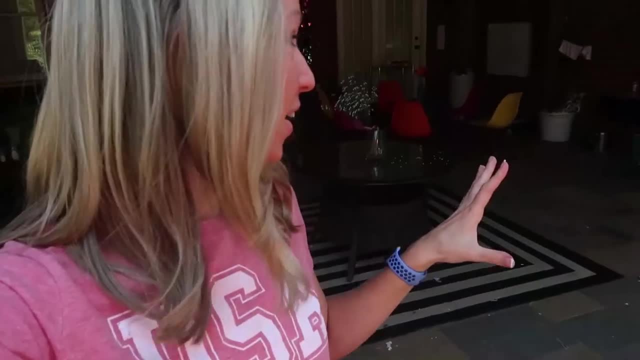 It's your own little lunch table And you made an umbrella. I see, Yeah, We found an old brick and we got some rocks, hot glued it, Wow. And then, if we come in here, they have pulled all sorts of furniture out of our storage. 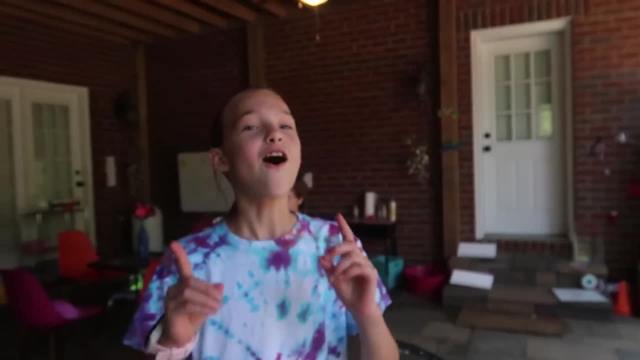 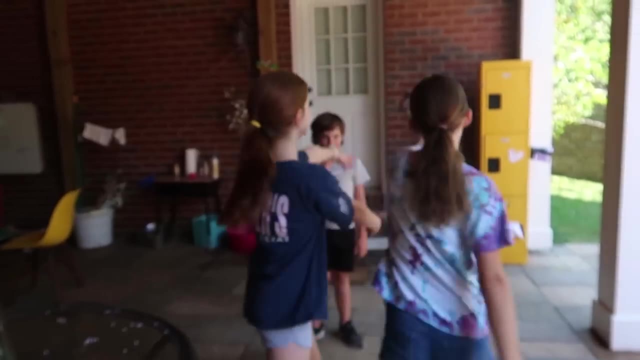 room out of pretty much everywhere. Yes, The hardest thing that me and Caroline had to lug from the storage room, What was it? Down the steps into the hangout and put back up our storage room. Oh my gosh, Oh my gosh. 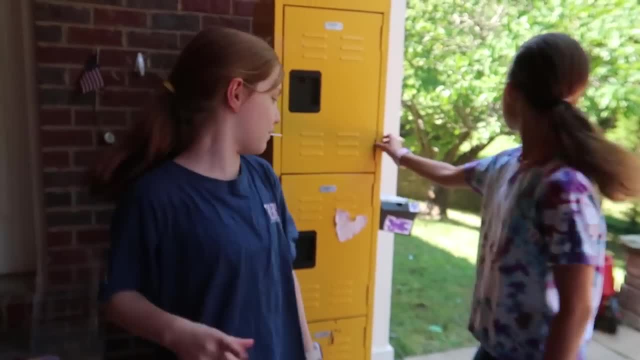 It was like a locker. Was this locker? No, it was just us, and we had to use the wagon to bring it down to the steps. Wow, And this was from our toy scientist set, wasn't it? This is my locker with Caroline's. 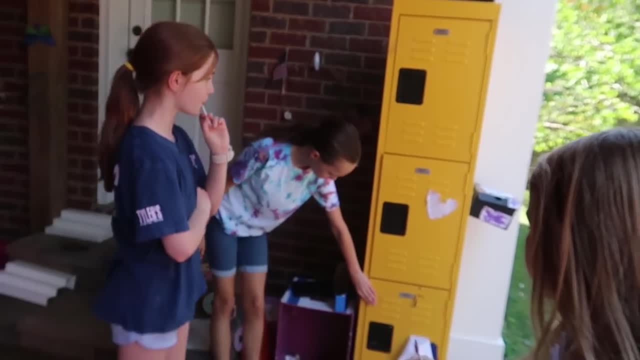 That's Maya's, This is Clark's and we're working on one for Emerson. This is our mailbox right here. Oh a mailbox. What is the S for Spy? Oh, your spy club. Very fun, I love the mailbox. 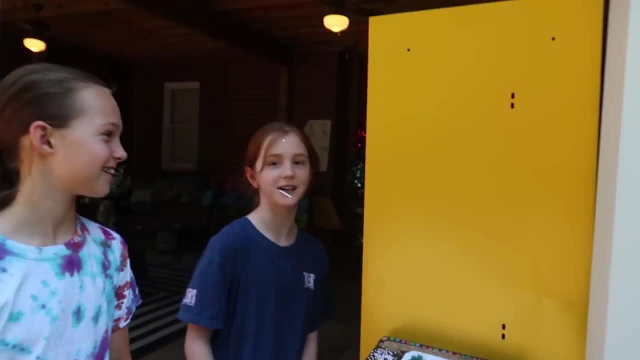 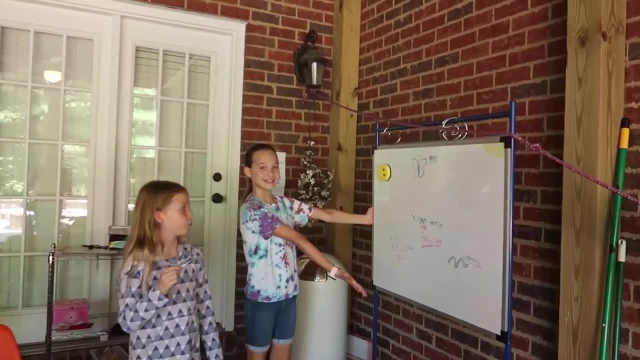 We have toys. We have toys. All these are huge pom poms. We're making one for each person. They're all going to be in the chairs. Oh, how fun. We've only made one so far. It's Addy's. 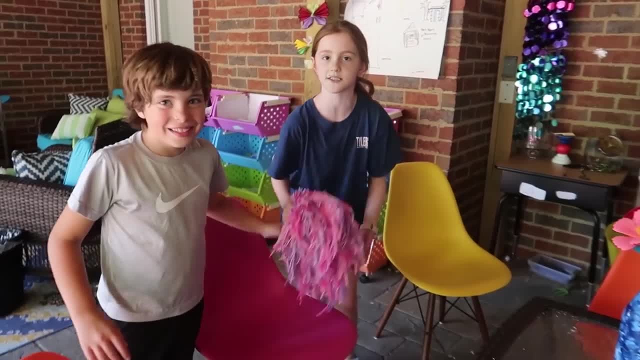 So cool. And what's this, Addy? This is from toy school And this is what you use for your meetings. Yes, And my favorite part of the hideout is over here: The candy table. The candy table, Wow. 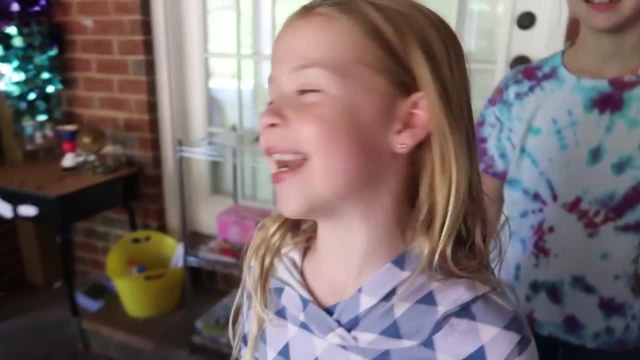 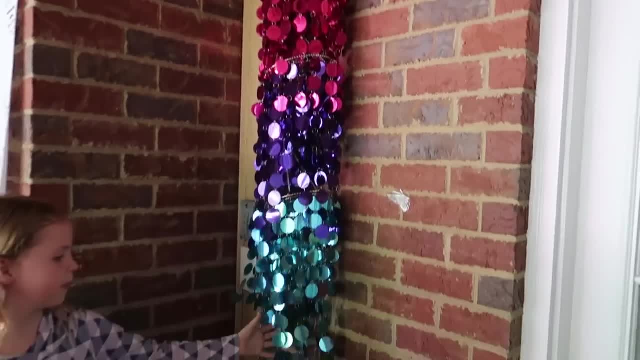 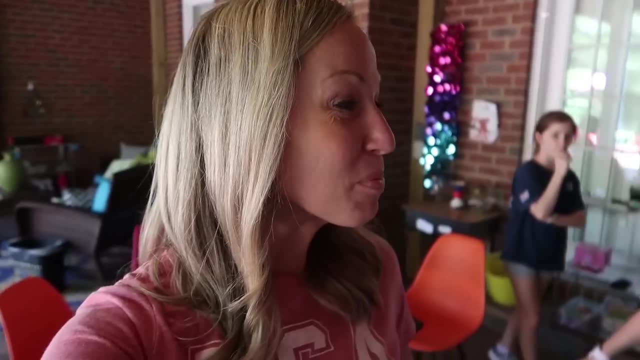 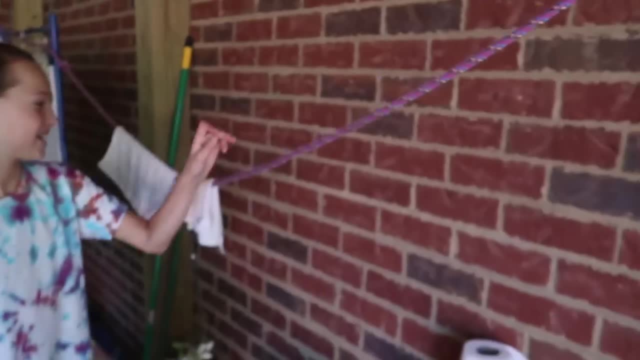 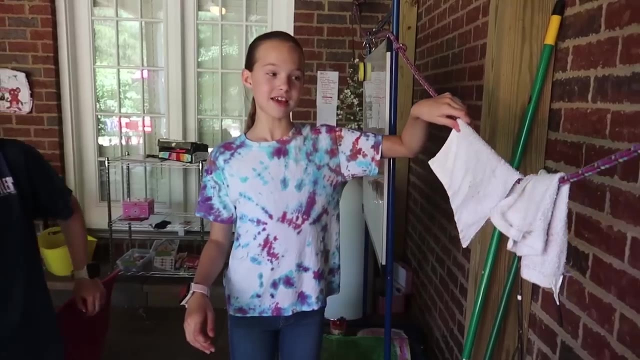 They're doing crafts all the time. What is this thing behind you? Oh, it's our clothesline. Your clothesline? Yeah, we do. We make this place really messy, so we have a clothesline so we can put our rags. that. 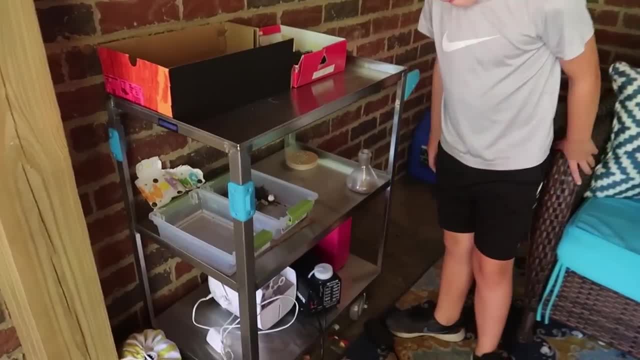 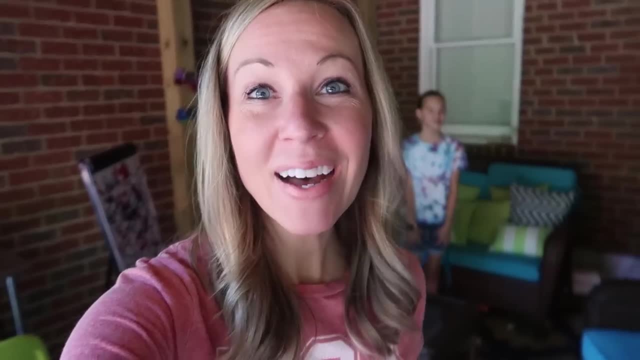 we help clean us with Wow And we have a worm farm. We don't know if they're dead or alive anymore. Worm farm- wow, And this is from Toy Hotel. right, That's our cart for Toy Hotel. Because of COVID-19,, the kids didn't get to play together. 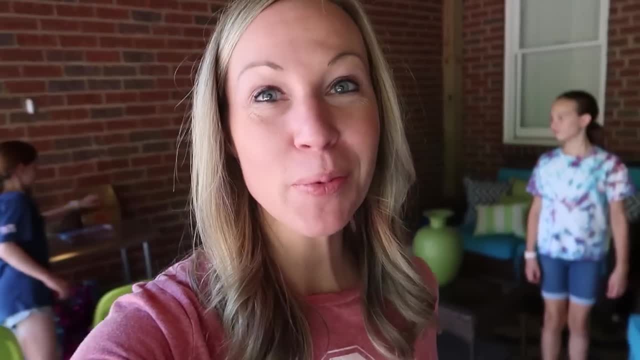 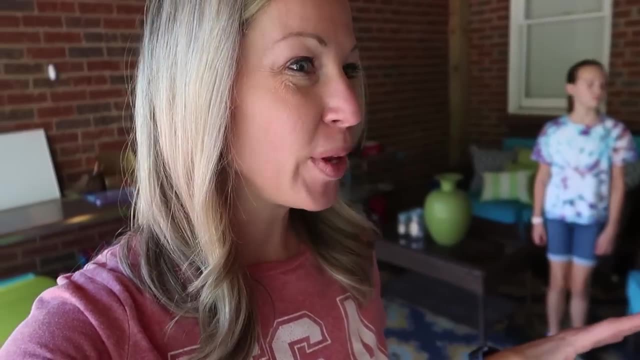 for months and they love their neighborhood buds. So more recently the neighbors and I decided that the kids needed to get together and for their own emotional health and mental health. so we decided the kids could play outside together but we wouldn't go into each other's houses. 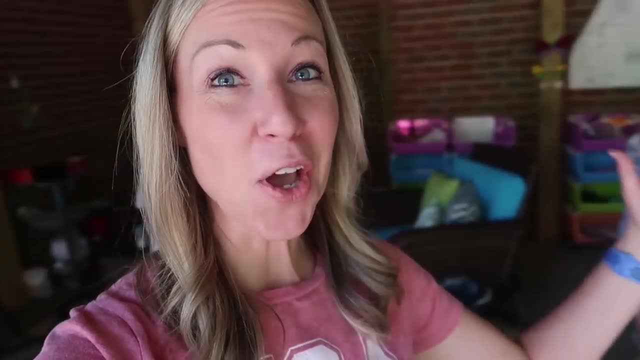 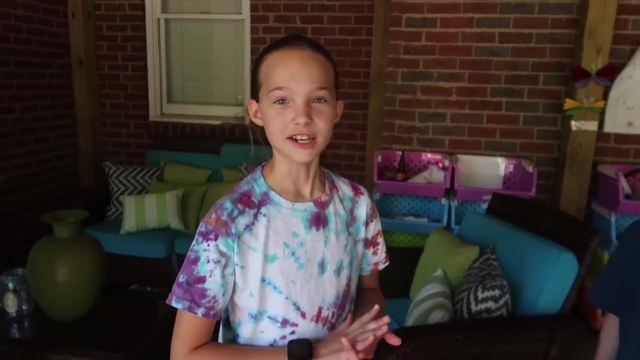 And since we can play outside, the kids have been doing all of this to keep themselves busy during the days. So why we created this hangout? Well, we got the inspiration from just eating lunch in here, From just eating lunch in here one day. 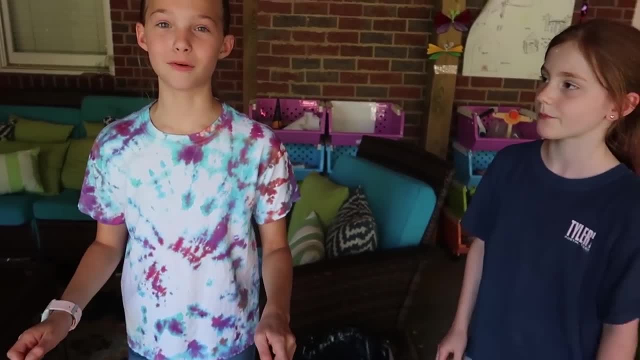 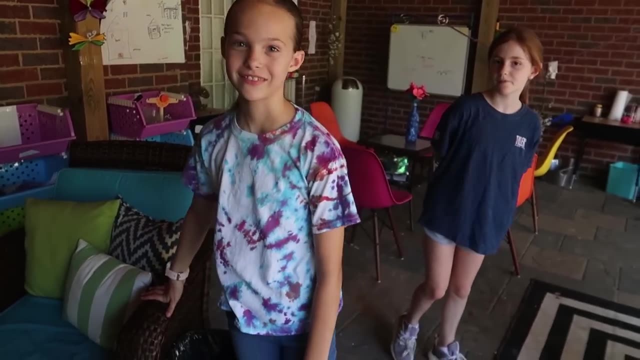 You turned it into a cool hangout. Yeah, the first day we got back from playing, cushions were all over the place. We have barely any of this furniture in here And you transformed it. Yeah, we put a couple of them together. 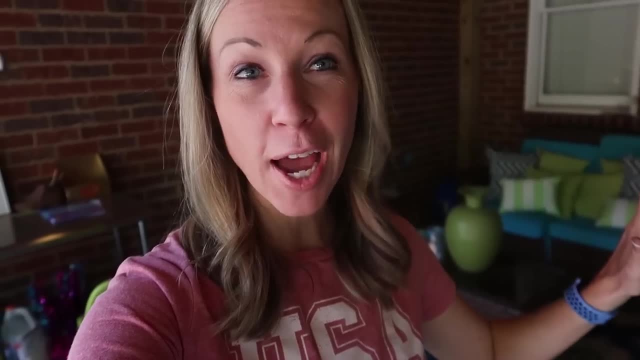 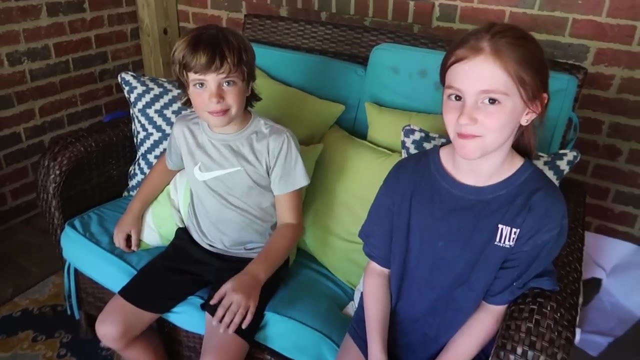 And two of their neighborhood buds that you've seen here, who are here all the time, pretty much every day, are Caroline and Emerson. Here's Miss Caroline and Emerson say hi, guys, Hi, And we have a few other friends too. but I'd say 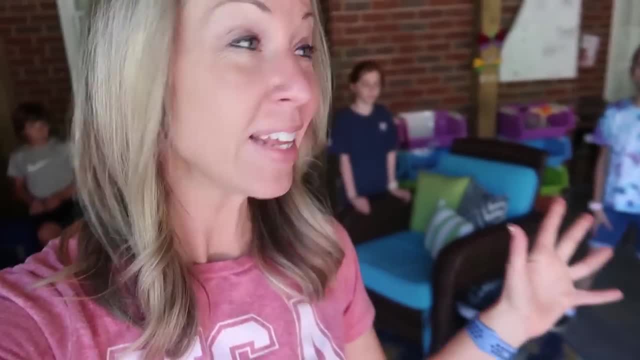 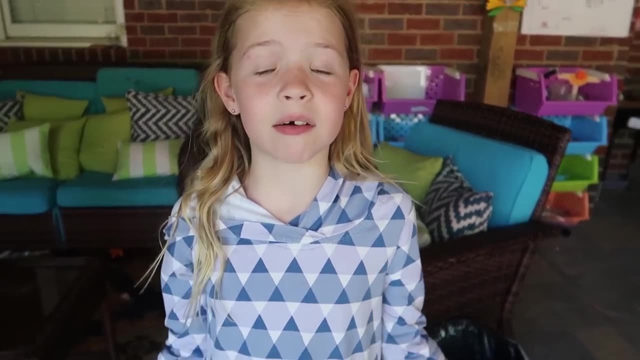 Caroline and Emerson and Clark probably are the ones who are here the most. Anything else you wanna show the audience about your cool hideout area? Sometimes we like saving up for stuff that we can put in here, So this is our needs, this is our wants, jar. 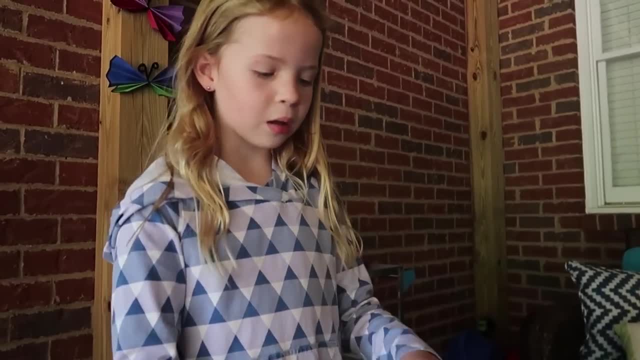 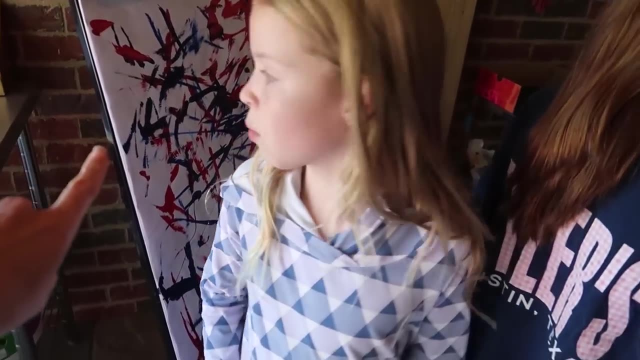 Oh, okay, so this is needs jar and wants jar. Also, you're saving money, And did you spray paint these too? it looks like I painted it with nail polisher. Very pretty, and I see you have some art over here. 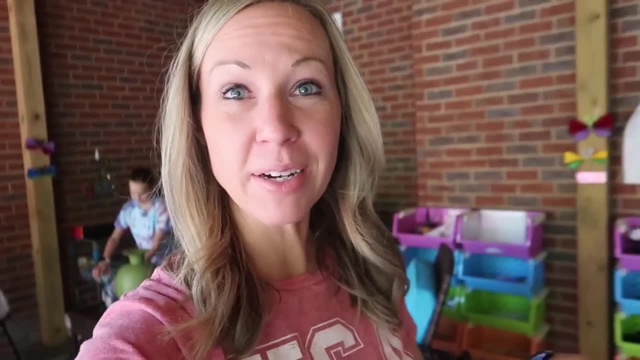 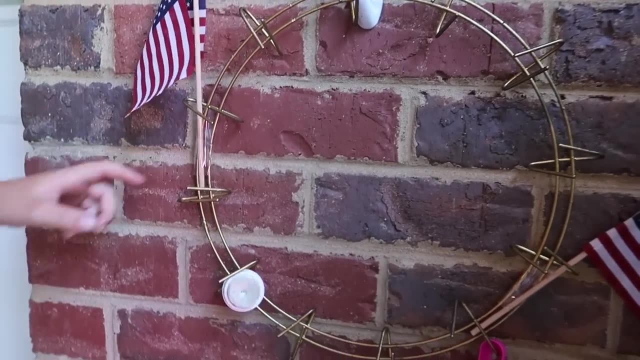 Oh yes, I did that to cover up our spy plans. And then Emerson has something over here that they've also been working on. What is this? We spray painted this and we can paint gizmos and all the watches and all that stuff. 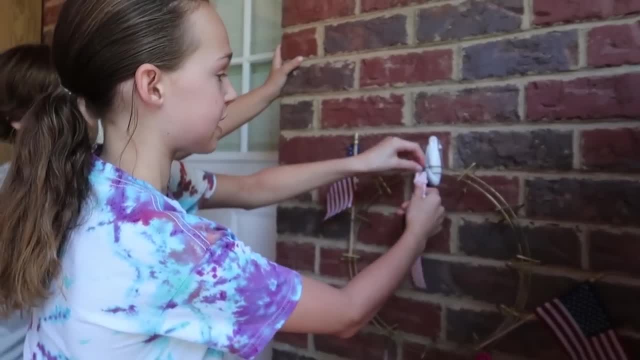 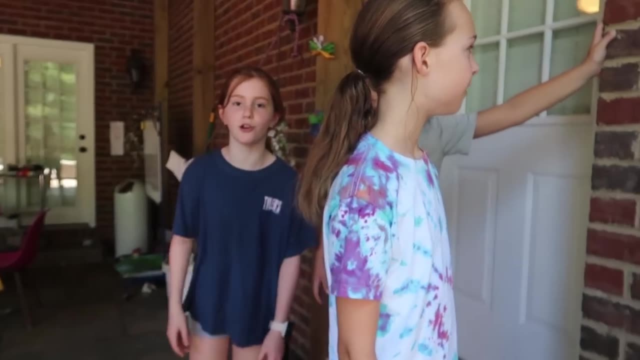 And what is that that you spray painted? Basically, we found it between mine and Emerson's backyard. It was a wreath hanger, but then we spray painted it gold from green. Yeah, I think someone just threw it in the forest and they didn't need it. 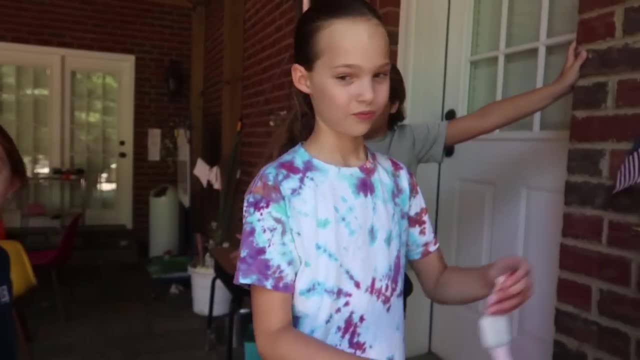 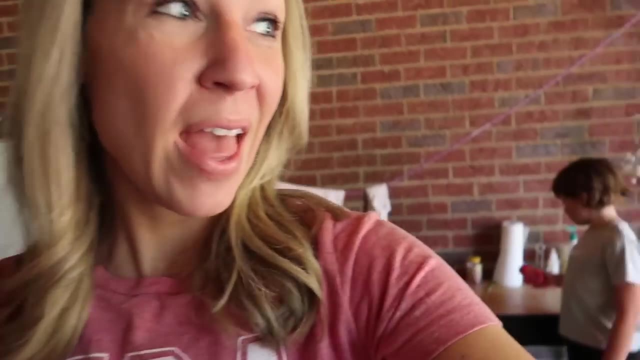 It was like garbage, but we turned it into something cool. I love it. You've been doing a lot of painting. We have a beautiful vase over here that they painted. Did you make this, Caroline? Yes, That turned out pretty. 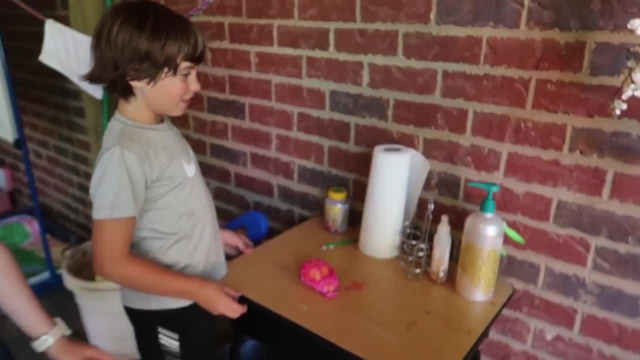 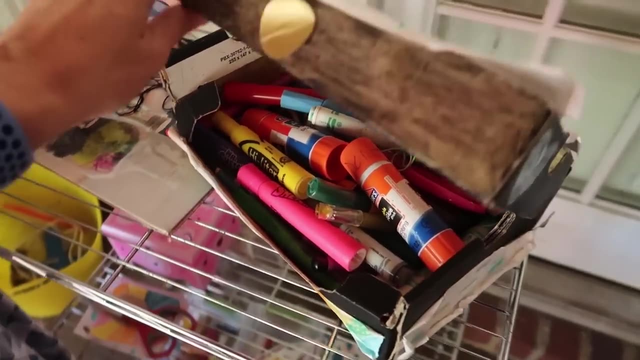 This is like that's going to be art. It's gonna be an art station. Yeah, we're gonna hang a few and we're gonna hang them. Oh, so fun Art supplies. And this is your craft box. Yeah, yeah. 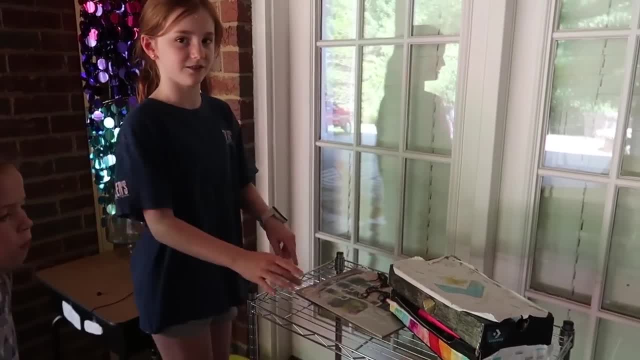 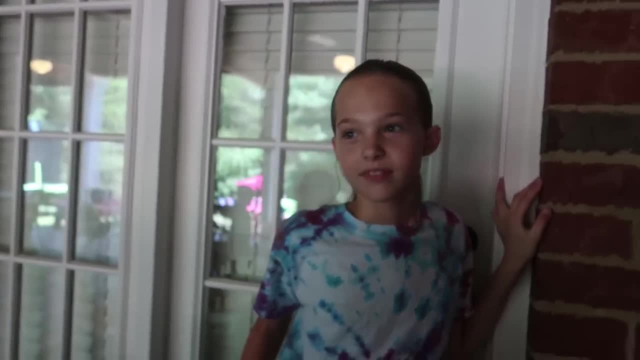 So you have all these art supplies you can work on. Yeah, I have an old shoe box and I made it all pretty. How cool Is this? a song list? Oh yeah, we like playing songs a lot, That's right. what else? 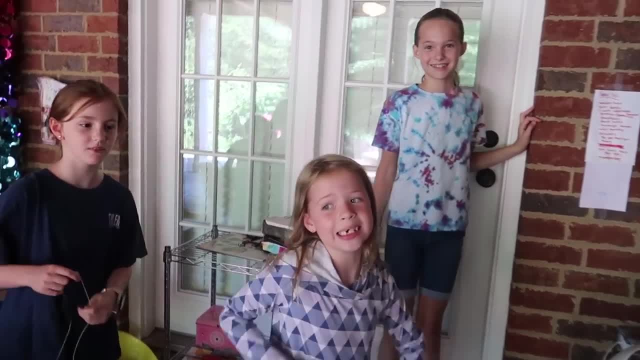 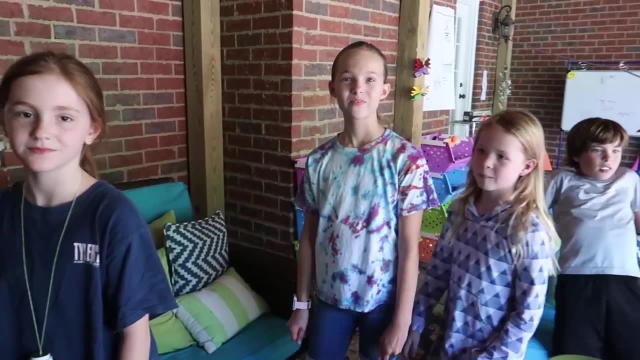 because what do you guys bring down here? a lot, This is Alexa. Alexa, Yeah, So you made art, you hung up and you made that. Caroline, Yes, You guys are so artistic and creative down here, Thank you. We make like music videos all the time. 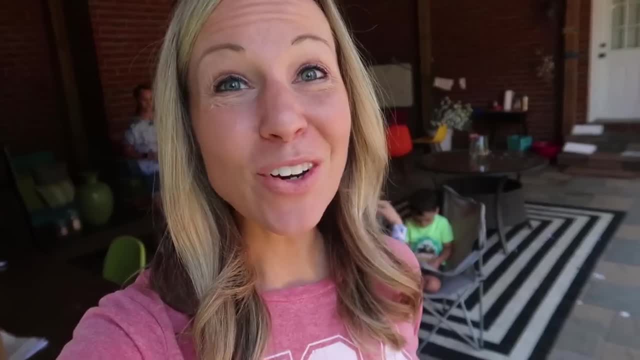 They do make music videos. Yeah, we made like the Queen of Mean music video. Well, I don't know about you, but I love their hideout. I think it's the funnest place and I love that it's done all by them. 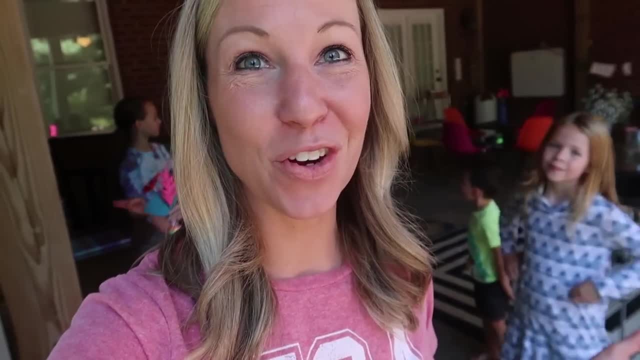 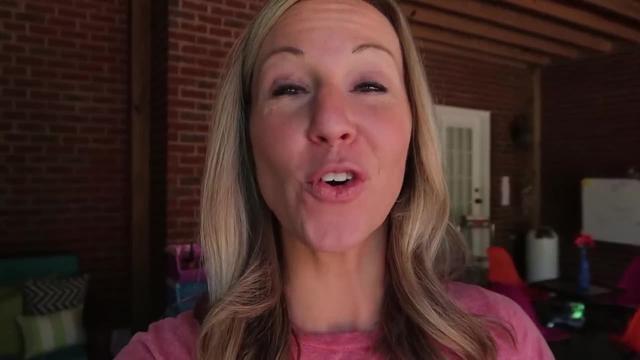 So much creativity has gone into this place and it's just fun to see all the creations that they've come up with. And you kiddos will spend hours down here, won't you guys? Yes, For hours at a time. In the summer we like asked each other to play at like 10 am.